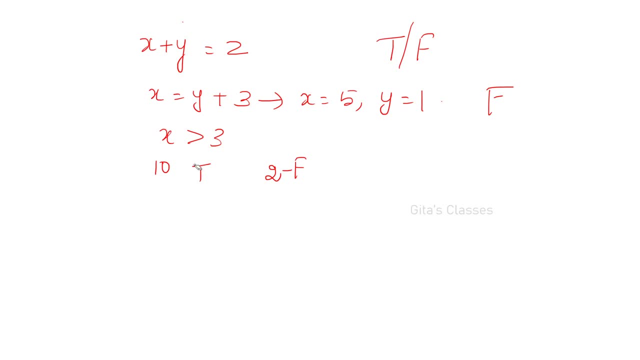 to 2 here, then it will become false. So, depending on the values, because it is a variable, we can't say that it is true or false, but we can make it true by assigning some variables. Okay, So this is the. 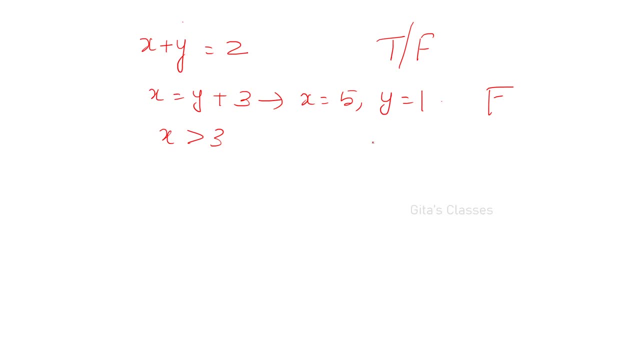 Predicate x. these kind of statements are predicates, right. So here x is called the subject and the first part. suppose, if you consider x is greater than 3,, x is greater than 3.. If you consider e is greater than 3, here the variable x alone is called the. 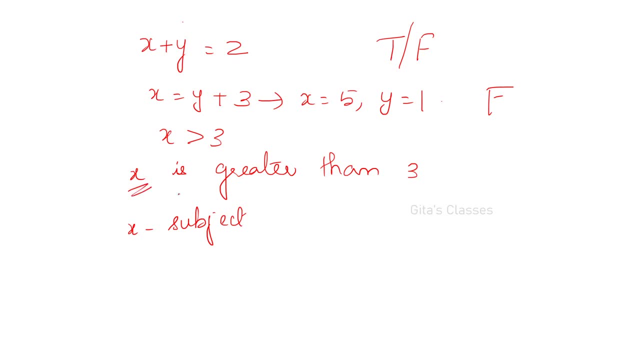 subject: The first part: x is called the subject And this is called the predicate. Okay, This x greater than 3 is the property that the subject of the statement can have. Okay, That is called. the second part is called the predicate right. 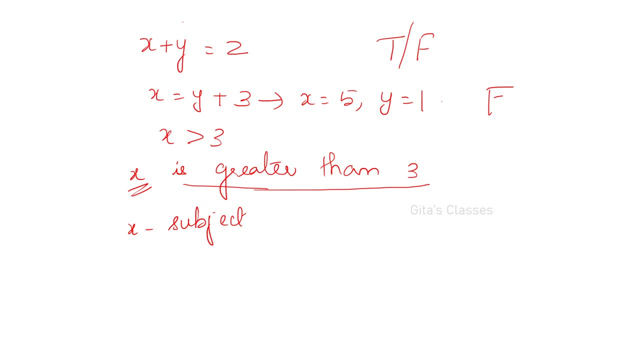 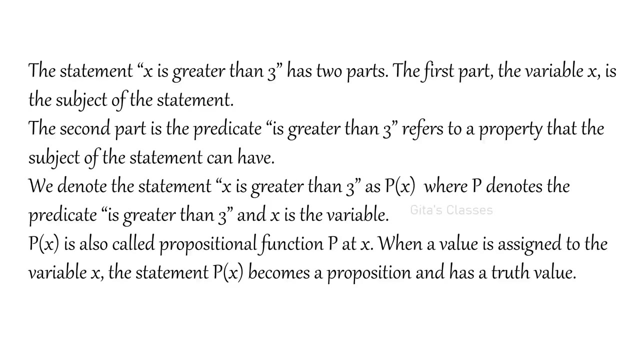 Quantifiers we will see soon. Now let us discuss these things, Then we will go to quantifiers. So the statement x is greater than 3 has two parts. You can go through this. The first part is the variable And it is called the subject of the statement. Okay, The second part is the predicate is: 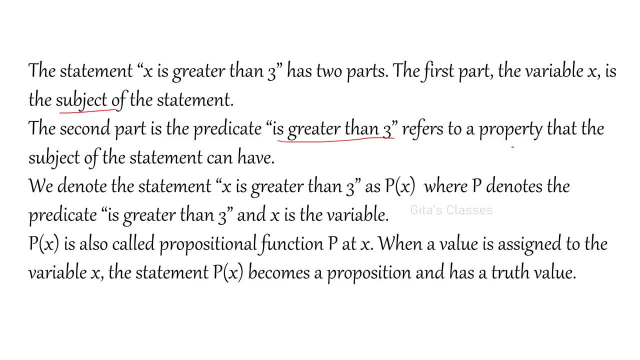 greater than 3.. This is what I have explained. now It refers to a property that the subject of the statement can have. Now we denote the statement as p of x, where p denotes the predicate is greater than 3 and x is the variable. So this is the predicate and we can have variables. 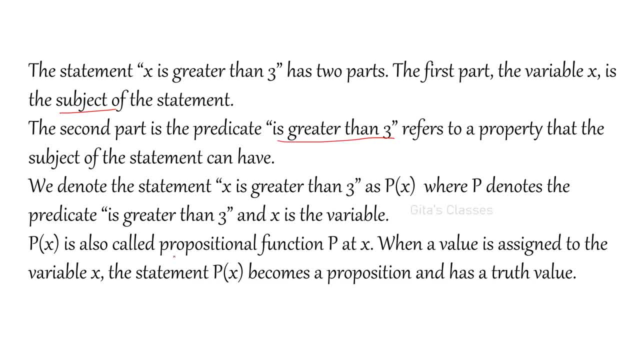 accordingly right. So p of x is also called propositional function, Another name for this. When a value is assigned to the variable x, p of x will become proposition and it has truth value. either It will become either true or false. 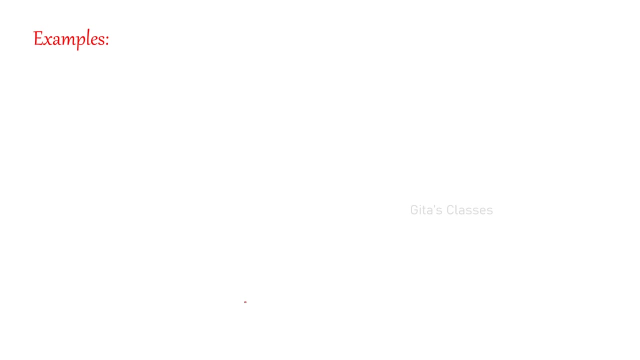 Let us see some more examples. Let q of x comma and one more part. if p of x is there only one variable, then it is called unary predicates. Unary predicate Cheers Ajay's speech predicate: if you have two variables- q of x comma, y or p of the same variable, also we can use p of. 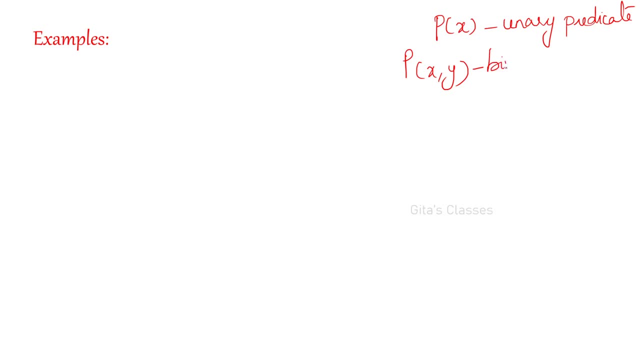 x comma, y. if you have two variables in this, it is called binary predicate. and if you have n variables- p of x1 comma, x2 comma- it can be extended to any number of variables. it is called n-ary predicate. so how many variables are there in this? okay, depending. 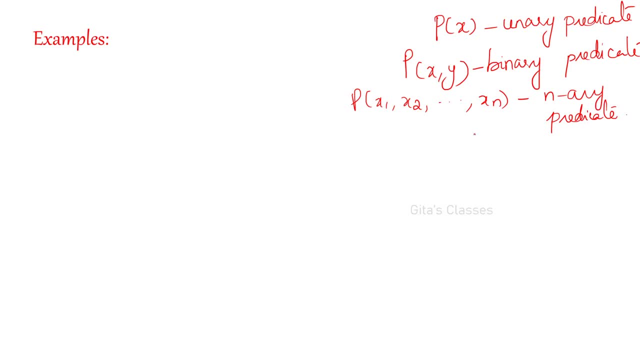 on that we give the names or n place, n-ary predicate or n place predicate. we can say: okay. now we'll see some more examples. q of x comma y is the statement, is the statement is the statement. x is equal to y plus 3. so what is the value of q of 1 comma 2? if i assign q, x is equal to 1, y is equal to 2. we 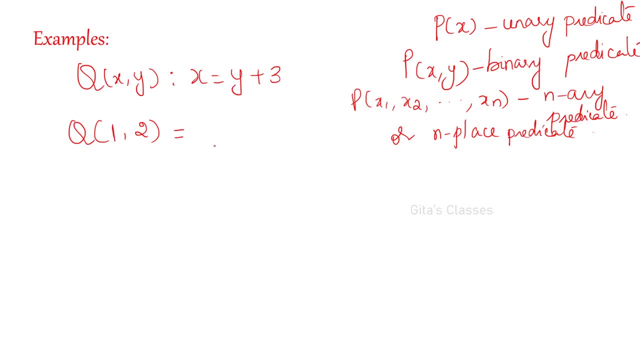 will write like this: q of 1 comma 2. okay, what is q of 1 comma 2? x will become 1. 1 is equal to 2 plus 3. what is the value? now we have assigned the values for x and y. it has become true or false. this has become: 2 plus 3 is 5. here we have written y. 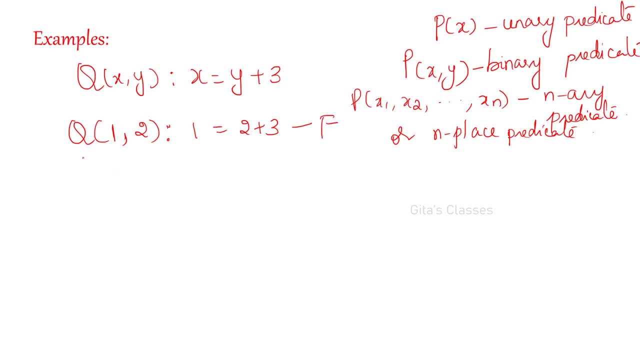 1. therefore it is false, right suppose? if i want q of 3 comma 0, what will be the values? x is equal to 3. i have assigned is equal to: y is 0 plus 3, so it will become true. okay, so by assigning the values. 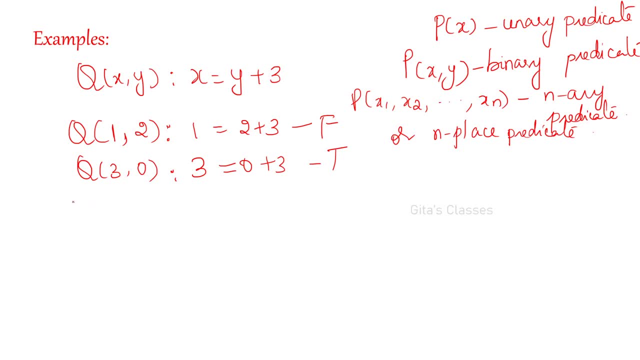 we can make it true or false. right next is r of. these are called predicates r of x, y. z is x plus y is equal to z. these are the statements right now. what is r of? can you say what is r of? 1 comma, 2 comma 3? 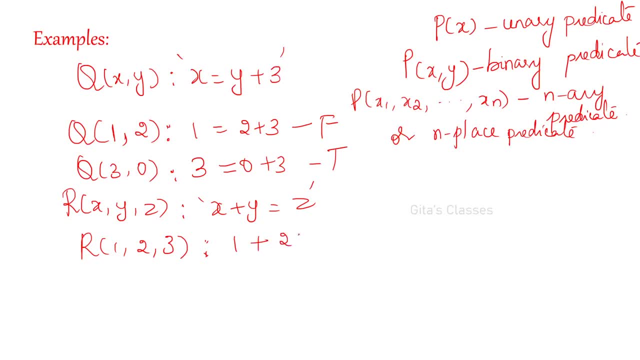 so 1 plus 2 is equal to 3. 1 plus 2 is equal to 3. therefore it has become true that's all. r of 0 comma 0 comma 2 is equal to 0. r of 0 comma 0 comma 2 is equal to 0. r of 0 comma 0 comma 2 is equal to 0. 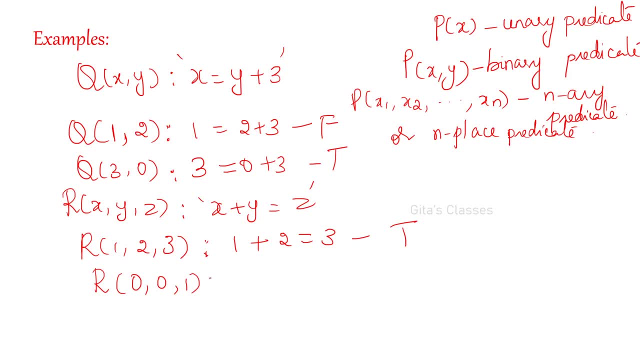 comma 1. what will be the value of r of 0 comma 0 comma 1, left hand side is 0 plus 0, which is equal to 1. it has become false. so by assigning the values, it will become true or false. okay, so these are the. 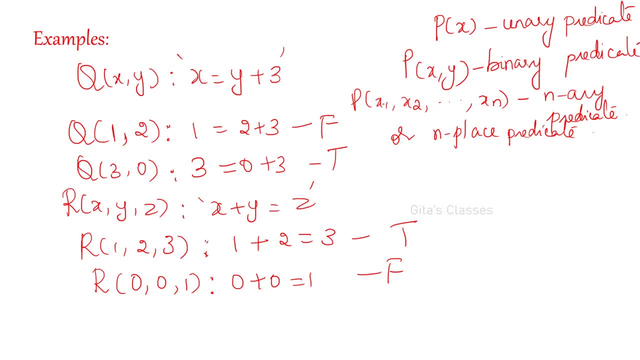 predicates p of x or p of x comma y or p of x, comma y, comma z. it need not be the same variable p. you can have q, r anything if you assign the way. these are the variables. okay, these are the variables. and the number. whatever number values are assigned to these variables, it will become: 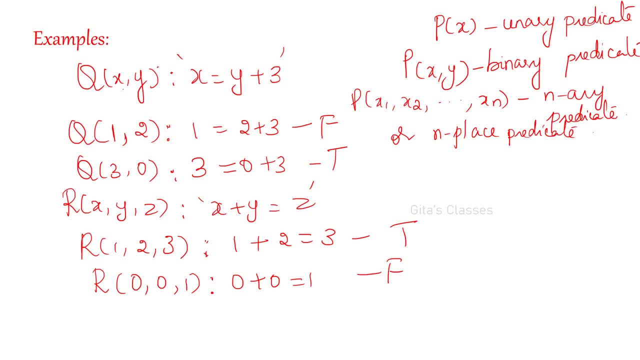 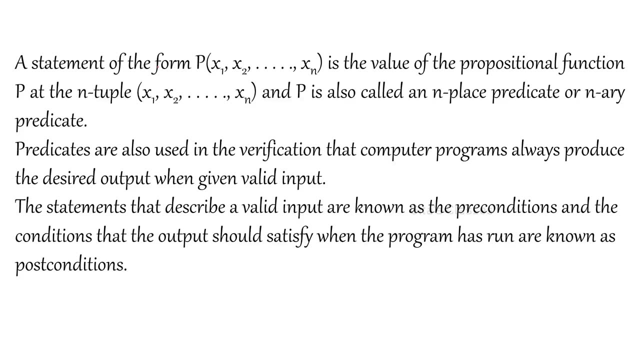 accordingly, it will become true or false. we can make the predicate true or false by assigning values to the variables. okay, so a statement of the form p of x 1 x 2 extra x n is the value of propositional function p at the n tuple, x, 1 x 2, etc. x, n and p is also called n place predicate or: 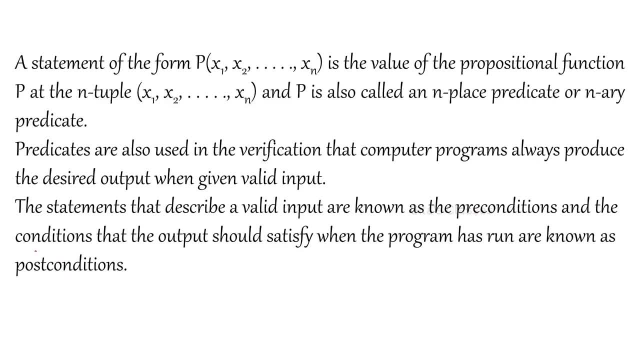 predicate and we are. we are having some applications of predicates also. predicates are also used in the verification that the computer programs always produce the desired output when given valid input. so before pre-conditions, that is, before running the programs also, we can check the values. after executing the program also you can check the values. so where values are correct. 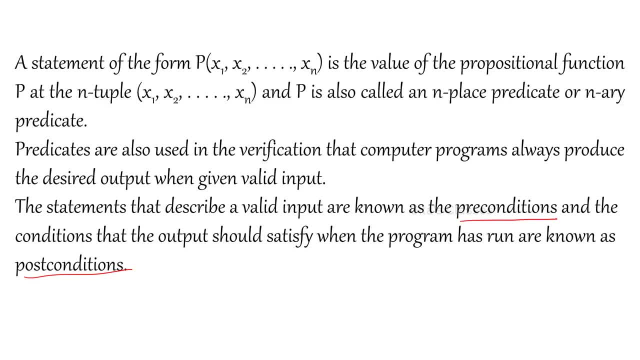 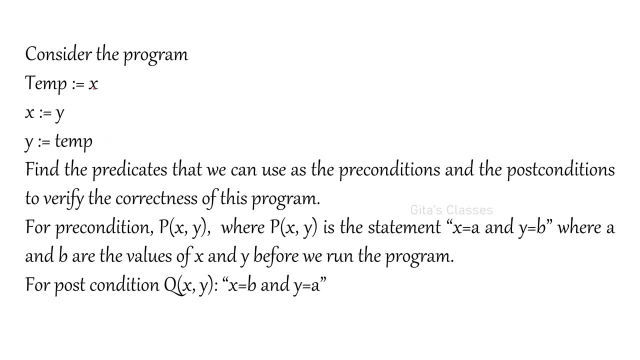 or not. so they are called pre-conditions and post-conditions. before executing the program, you can check the values. you can have the check you. for that we can use. this predicates okay how we'll see one example. consider the program: temporary value is equal to x, x is equal to y, y is equal to. 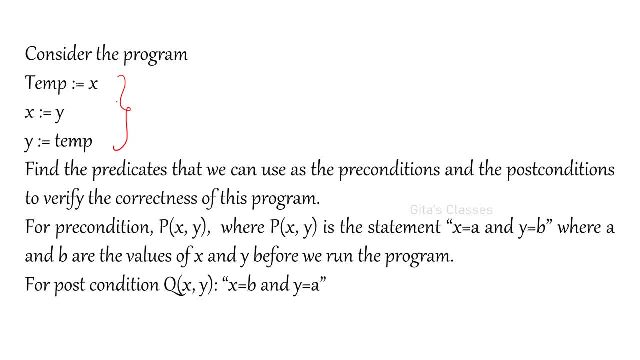 temp. all of you know what is this program that is just interchanging the values, right? so how will you use this? find the predicates that we can use the pre-conditions and post-conditions to verify the status of this program. so what will you check? suppose, if you are assuming some values? x is equal. 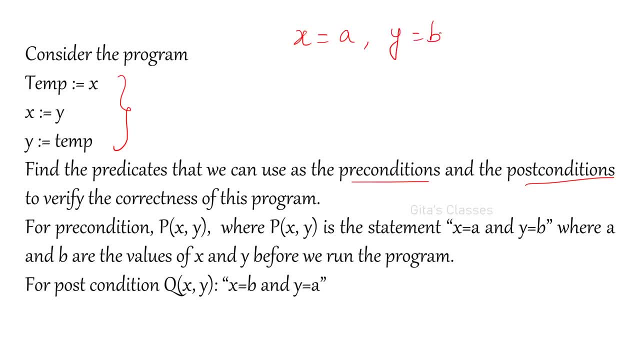 to a, y is equal. these are the initial values you have. so pre-conditions, you can write p of x comma y. okay, it is the statement: x is equal to a, y is equal to b. so this is our p of x comma y. this is for pre-conditions. so q and after that post-condition, after executing the program, what? 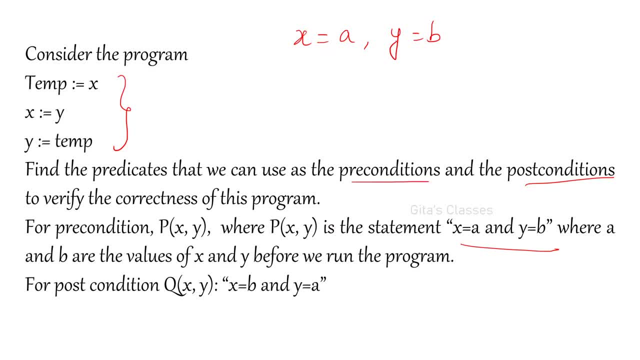 is the program objective. we have to interchange the values after executing the program. we have to, so what will be the output? this is the input, right? so input is x is equal to a, y is equal to b. what will be the output now? so you have to interchange, so x will become. now we have stored. 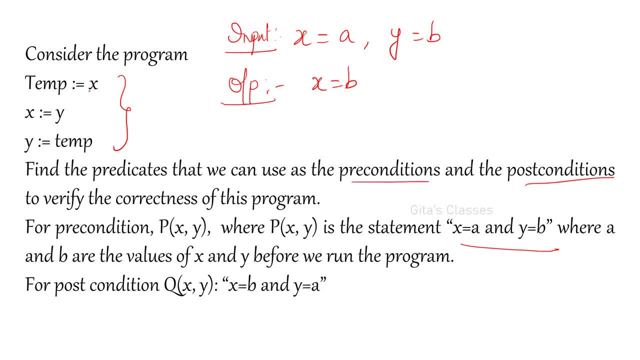 the value b in x, c, temporary. what is the? how will it execute? temp is equal to x. x value is what a right now. x will become y. value is what b. now y is equal to temp value a. so, after executing the program, x is equal to b, y is equal to e. so this, we are going to take it as. 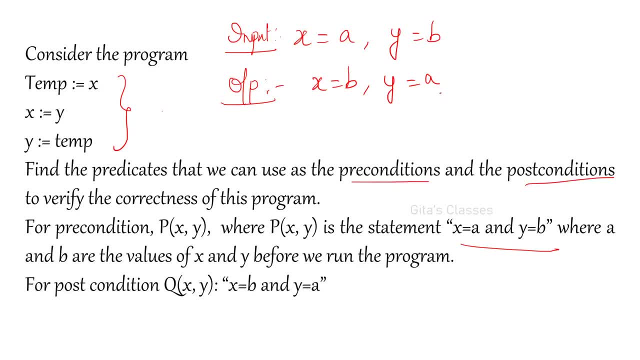 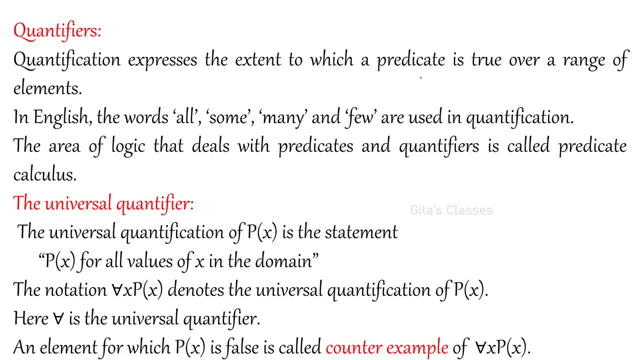 q of x comma y. we are going to check this. so for checking these programs conditions we can use predicates. okay, so next is another important thing: quantifiers quantify from the name itself. you can understand more. predicates is the. now we have seen i think i hope you would have understood. 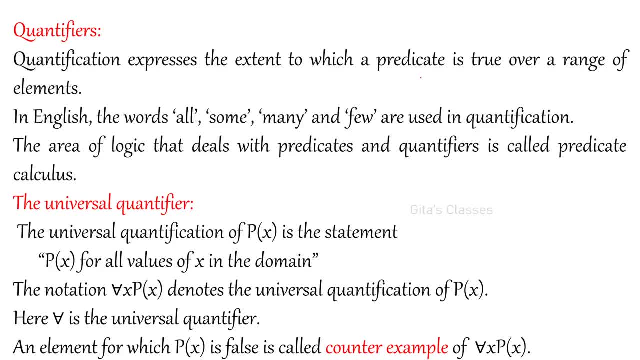 what is a predicate? so predicates will have some variables. for the variables you can assign some numbers or some values, depending on the values you are making the predicate- true or false. you are making the predicate statement, you are making the predicate propositions. okay, so as it is, it will not be. 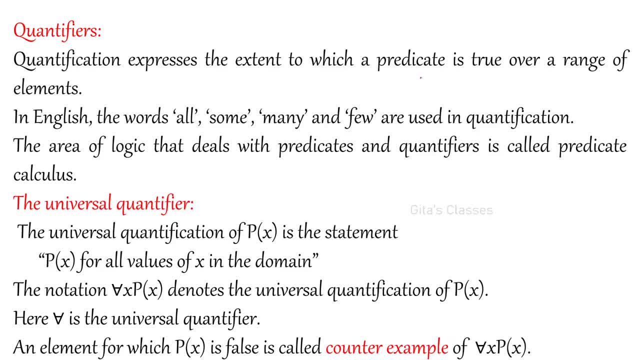 proposition. by assigning some values for the variables, it will become predicate propositions or statements. now to some: to what extent you can assign the values. if you assign some values: p of x, comma p of x. we have written: x is greater than 3. for what, for this x, what values can be assigned? can you assign a some name for this? 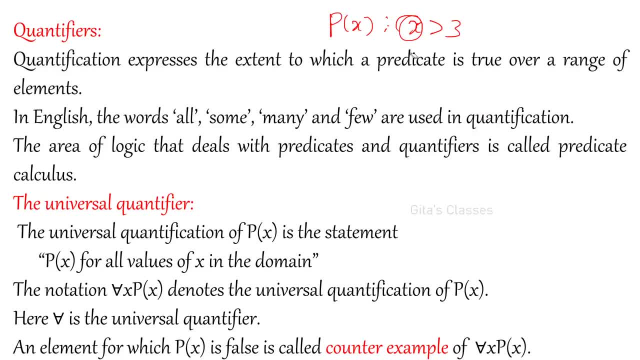 we can't now. okay, we have to assign some integers or real numbers, something like that. only we can assign to make it true or false. okay, you cannot assign some name. ram is greater than 3, can you assign like that? no, we can't. okay, we cannot compare now, we cannot make it true or false. so proper values should be. 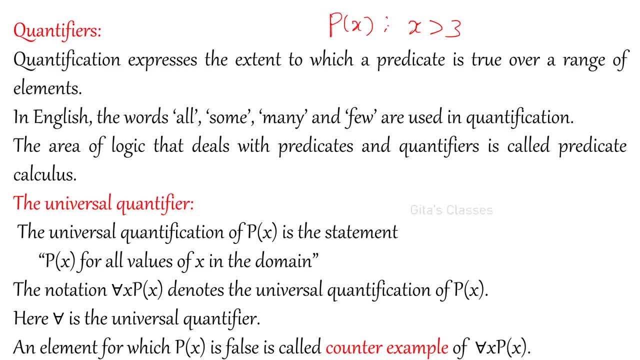 assigned for x, from which set you are going to assign these values. that is called quantifiers. that is, that defines the quantifiers. okay, so quantification expresses the extent to which a predicate is true over a range of elements. so in general we have- in english, we have all some- 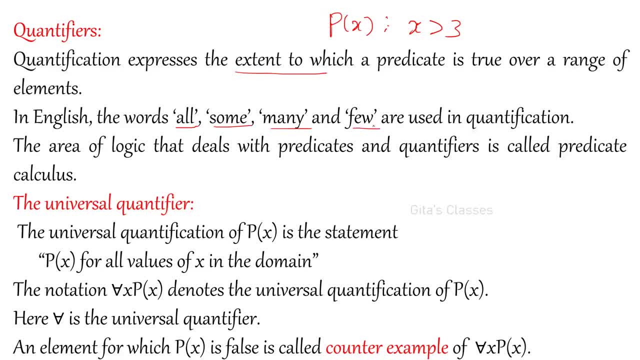 many few. these are all the words we are going to use for quantification. right next, the area of logic that deals with predicates and quantifiers is called the predicate calculus. so next we have some. what are all the quantifiers we can have? we have mainly two quantifiers: universal quantifier and existential quantifier. one is 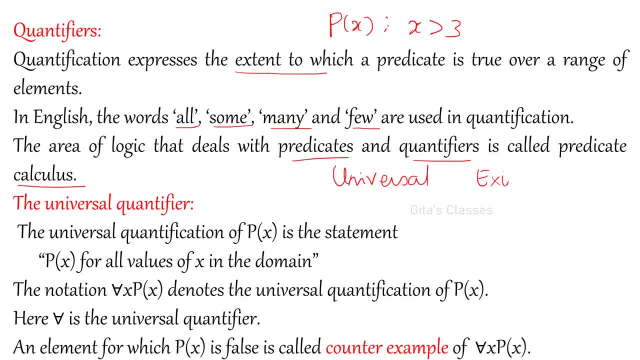 universal and existential. even from the name itself you can easily understand: universal means for all the values. existential means there exists some value. okay, from the name, try to remember universal quantifier. so universal quantification means p of x for all values of x in the domain. what do you mean by this? 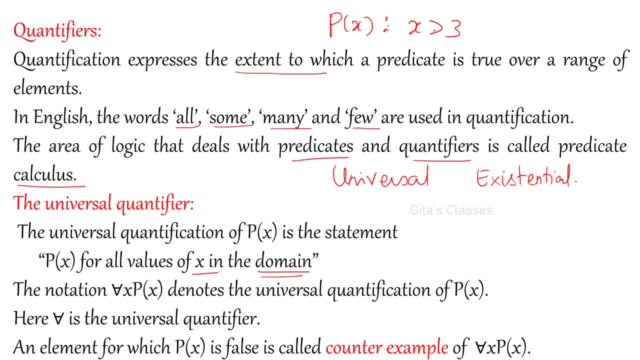 domain, see p of x. is x greater than 3? i told x can be a real number. so the set of real numbers is called the domain. okay, it is called the domain. and it can be set of integers. it can be set of real numbers- okay. set of natural numbers, set of whole numbers, anything. you can assign any value, any. 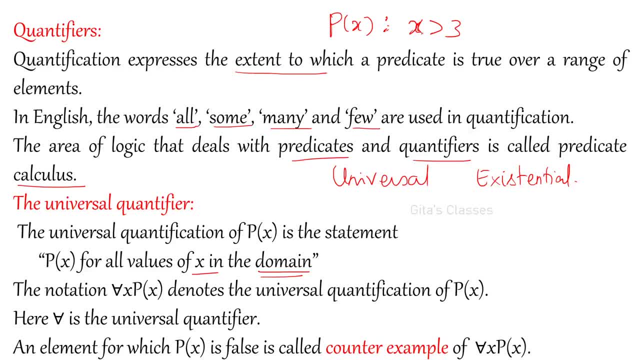 you can define the domain, you have to define the domain. if you are defining a predicate, definitely you have to define the domain also. okay, so the notation for all x, for in the domain, for all x, p, x denotes the universal quantification of p of x and here, for all is always: this is the notation for. 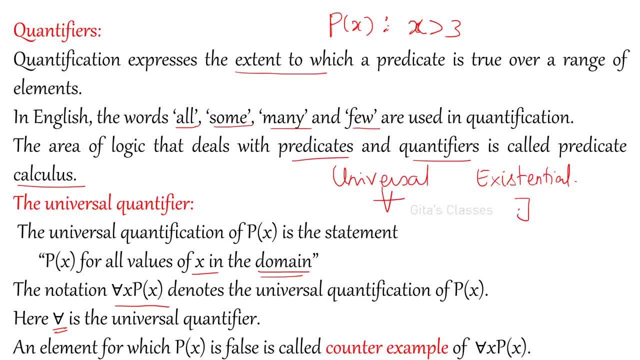 universal quantifier for all There exists, means existential. So an element for which p of x is false is called counter example. So if you can prove that somewhere, for at least if you are able to find out, there is some statement given for x, p of x, So now you can define whether it is true. 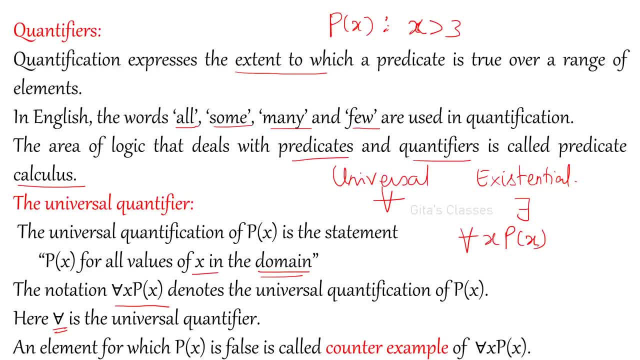 or false If for all the values you know, see, for example, if I give x is greater than 3 p of x, if I consider this statement, x is an integer, So if I am defining the domain as the set of integers, then I can give this is false. I will say: If I write for this statement, if I write for all x, p. 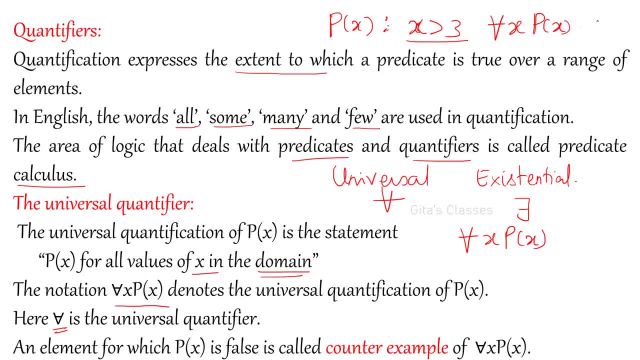 of x where p of x is x greater than 3. how will you say this? it is false. How can you say that you should be able to give one counter example? What is the counter example? if I assign x is equal to 5, x is greater. 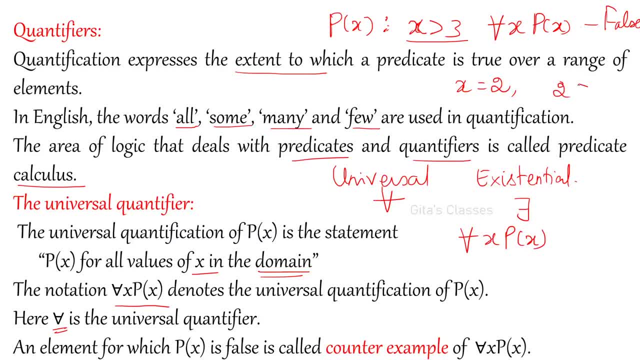 If I am giving x is equal to 2, then 2 greater than 3 is false. we know. If I am assigning x is equal to 5, it will become true. So for all values of integers, even if I assign x is equal to minus. 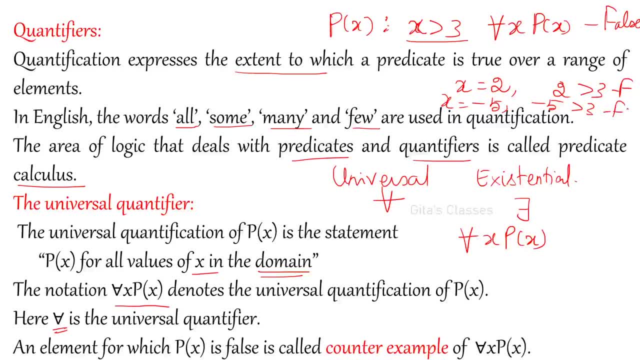 5 minus 5 greater than 3 is also false right. So if you can prove, if you can give at least one value for which it is false, then it will become false right. So it is not true for all the values of x right. 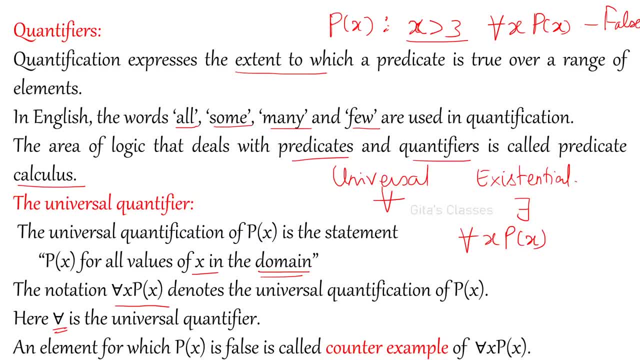 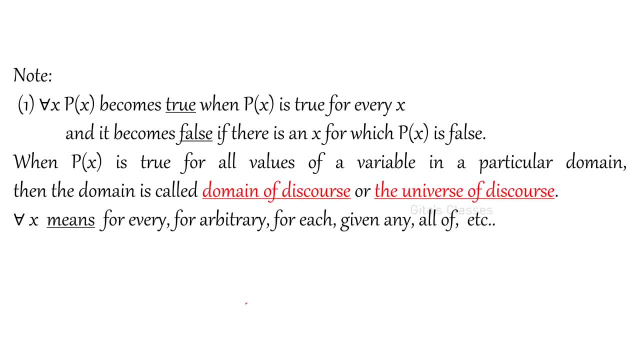 So counter example is: if you can prove that an element for which p of x is false, it is called the counter example for all x, p of x. So it will become true when p of x is true for all the values of x. it will become false if there exists at least one x for which p. 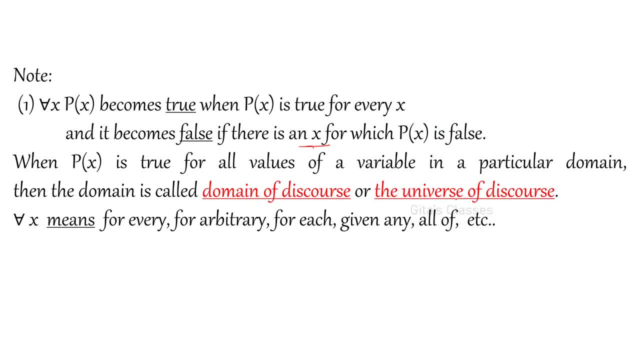 of x is false, ok, And p of x is true for all values of a variable in a particular domain. Domain is the set. Then the domain is called domain of discourse or universe of discourse, For here for all x means sometimes we will have for every. these are all the alternative. 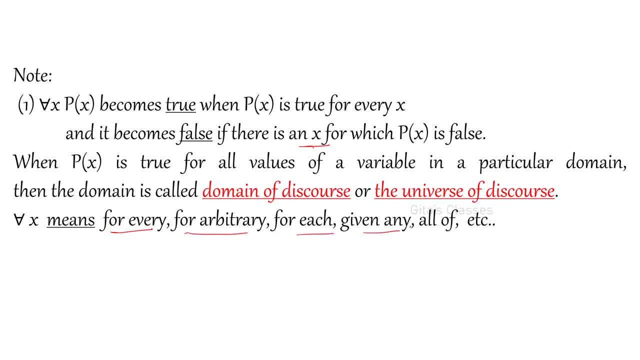 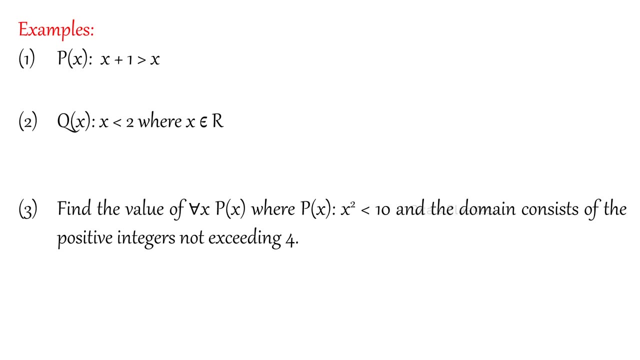 words we can get for arbitrary, for each given any. all of all these words are for for all, x only. ok, They may not give in the symbol sometimes. for all for every, like this, if they can give. Next we will see some more example. p of x is. p of x is the statement: x plus 1. 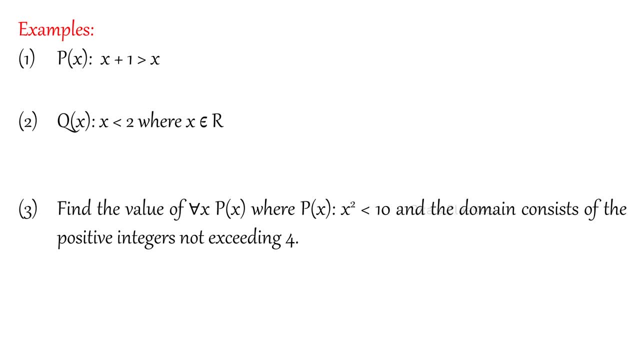 is greater than x. So what is the set? if the domain is the, and whenever you define this statement you have to give the domain also. Domain should be mentioned. What is the domain here? if the domain is set of real numbers, Set of real numbers, then then it will become for all x. 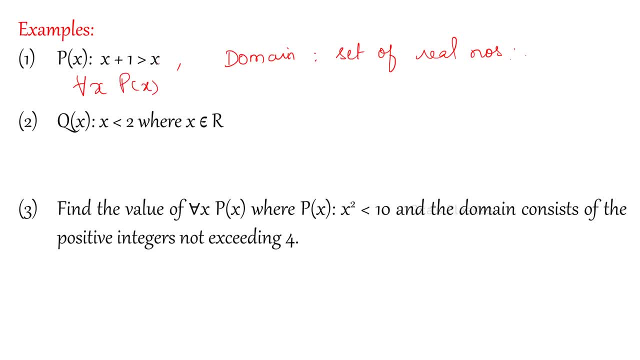 p of x is always greater than x. right x plus 1. what is p of x? x plus 1 is greater than x only. So if it is a set of real numbers- x plus for all x- p of x will become true, Even you can. 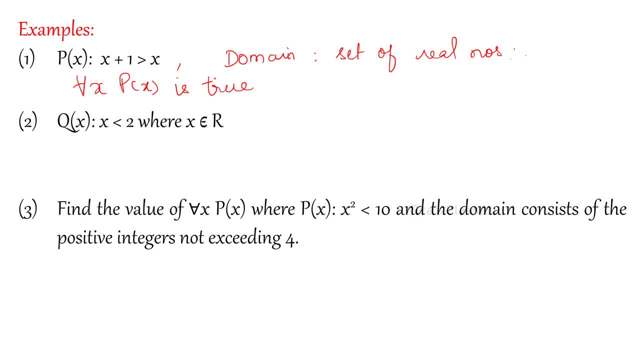 expect questions like this also. sometimes they will give some sentences. you will be asked to find out what is the value, whether it is having true or false value. Now, q of x is equal to x is less than 2, where x belongs to r. If you, if you write for all x, q of x. 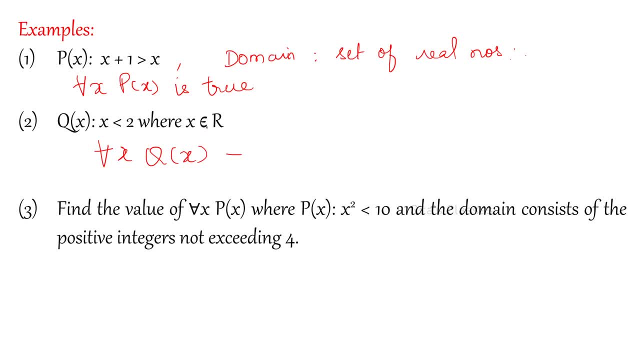 then it will become x is x is, x is any real number. therefore it will become false. Counter example: whenever you are telling for all x, q of x, then it will become false. you have to write So: false means counter example. you have to give What is a counter example. 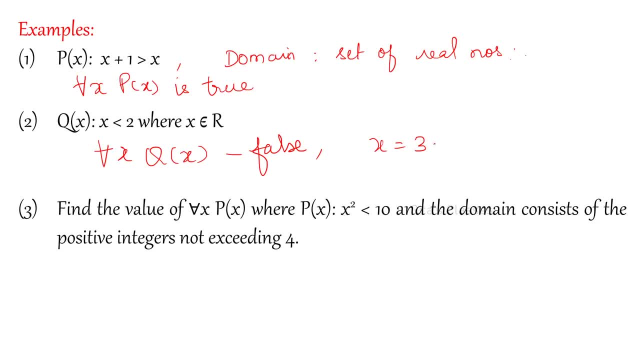 x is equal to 3 if you give. that is also a counter example, But it will become if there exists. Next we will see there exists x, q of x, Then at least one value from the domain we can find out, that will become true. ok, So 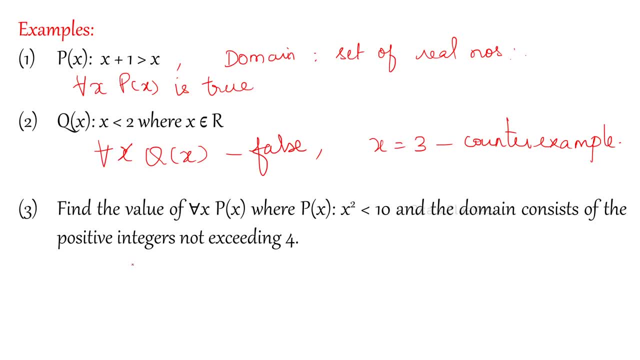 here now we are seeing only universal quantifier. Find the value of for all x, p of x, where p of x is greater than p of x, is x square is less than 10 and the domain consists of domain is defined as positive integers not exceeding 4.. So what are the positive integers not exceeding? 4.. So we have p of 1., p of 2., p of 3., p of 4., p of 5., p of 6., p of 7., p of 8., p of 9., p of 10., p of 11. p of. 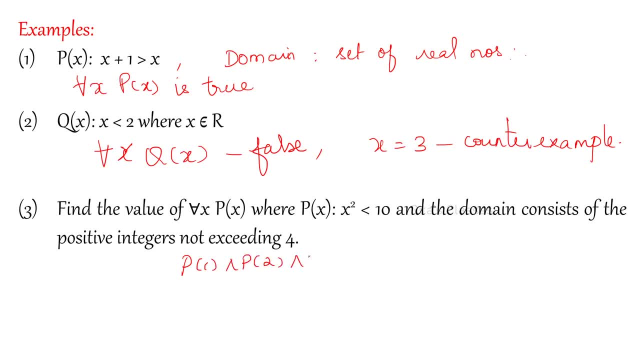 12, And then there are p of 1 and p of 2 and p of 3 and p of 4.. Okay, So these are the values. Now can you say whether it is true or false? p of one one square is less than. 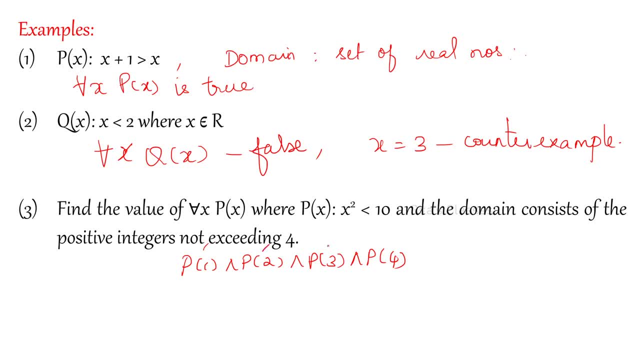 10, this is true. p of 2, it is true four. p of 3 is 9.. x square is three, square is nine. less than ten, true, But p of 4, it is 16, it is not less than So. at least one value it. 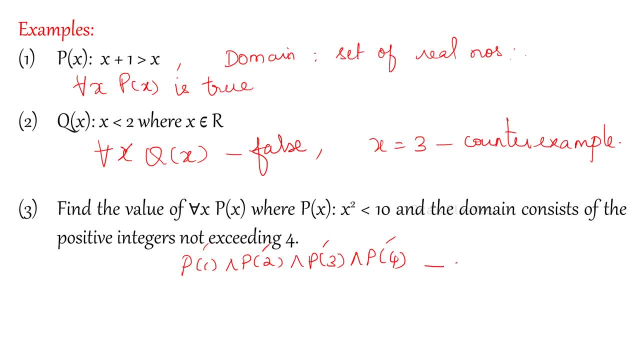 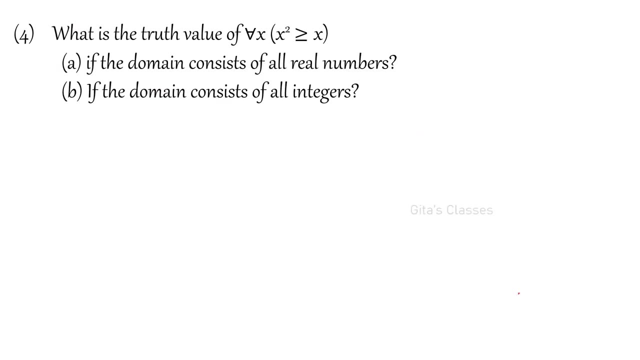 is not true is false, then it will become false Because p of 4 is false. We have given one counter example. We have one more question: What is the truth value of for all x, x squared greater than or equal to ex, if the domain consists of real numbers For the same variable, same predicate? 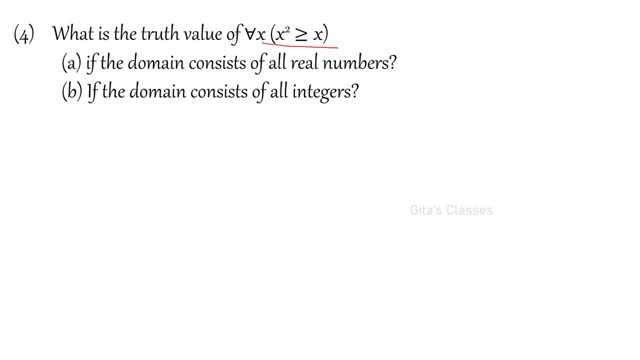 you can give different domains also. That's why I told you domain should be mentioned. Then only we can make it, We can understand whether it is true or false. So here, first one is: domain consists of real numbers. Real numbers means what? If you can, I can give you one counter example for 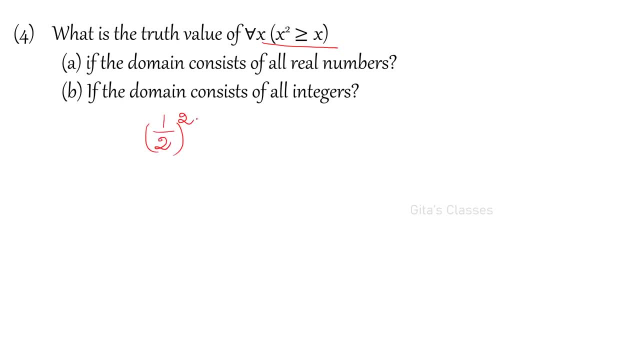 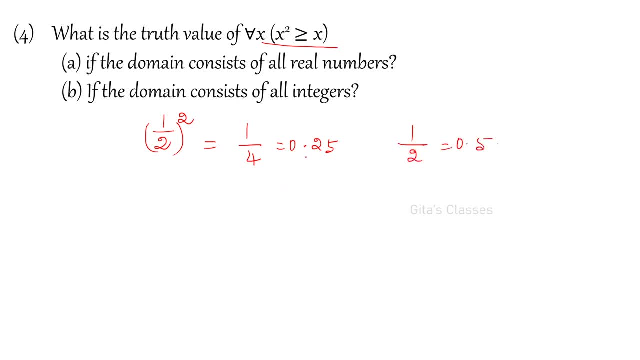 1 by 2 is 0.5. So 0.25 is not greater than or equal to 0.5. Therefore it will become false. So for the first one it is false. Therefore, x squared is greater than or equal to x only if. 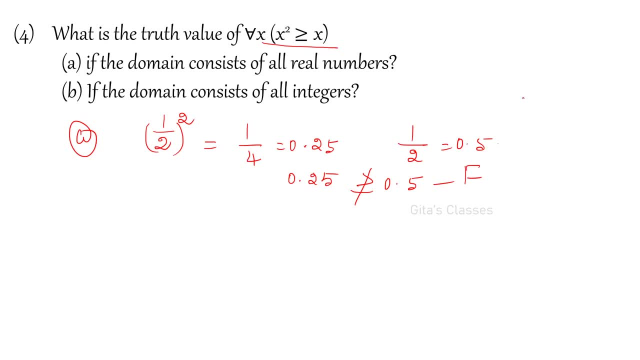 it should be less than or equal to 0.. In this interval, in 0,1,, it will not be true. So the if you can give one counter example, it will become false. So for this first one, the truth. 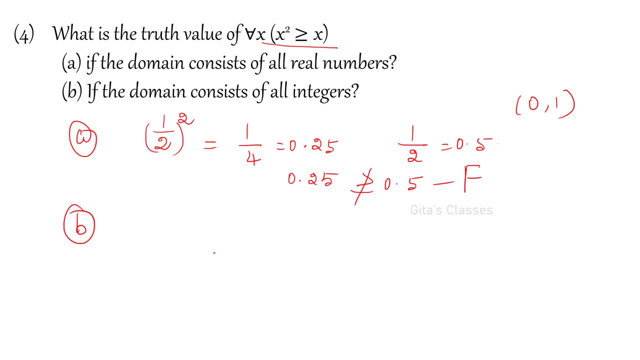 value of this will become false. Answer is false here. Now second one, for integers: domain Integers, domain x squared is always greater than or equal to x for all integers. Therefore it will become true. You are asked to find out the truth. value only. Next is existential. 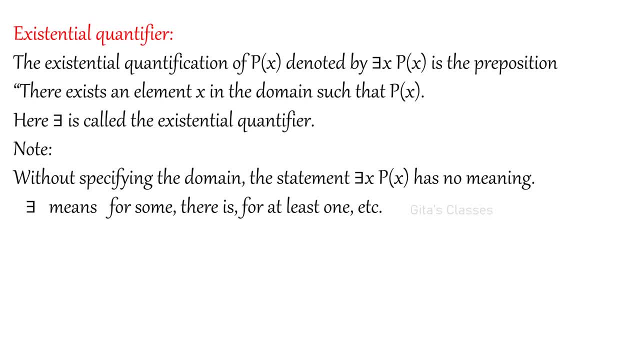 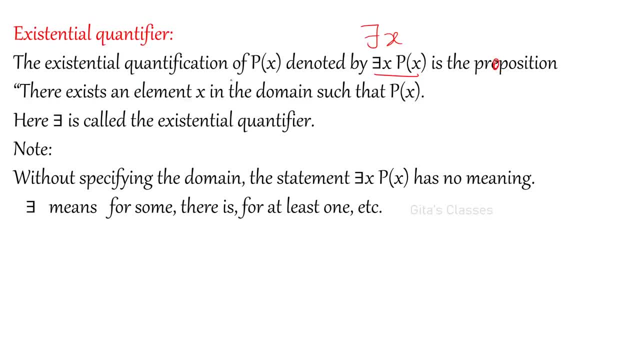 sorry, It is proposition. There exists an element x in the domain, such that p of x. So if you can find out at least one value in, then it is called existential quantifier. So if you can prove that this is true for at least one value, this will become true. 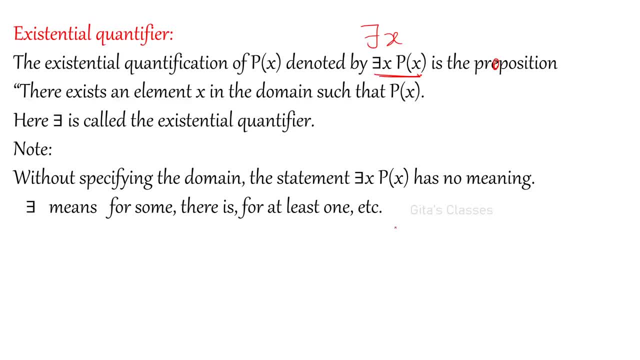 So without specifying the domain, the statement has no meaning. So there exists means for some and always- it is not not only existential- even for universal Domain should be mentioned. The statement there exists p of x means which x we have to take, we do not, we will not. 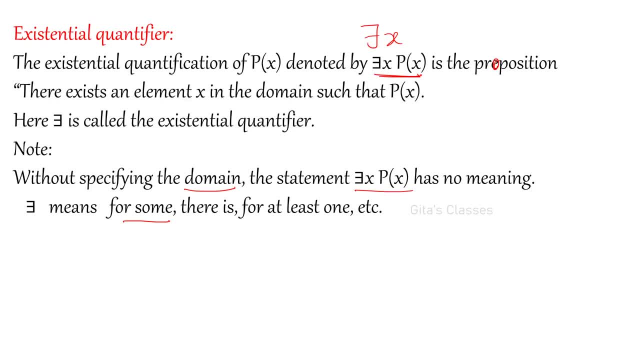 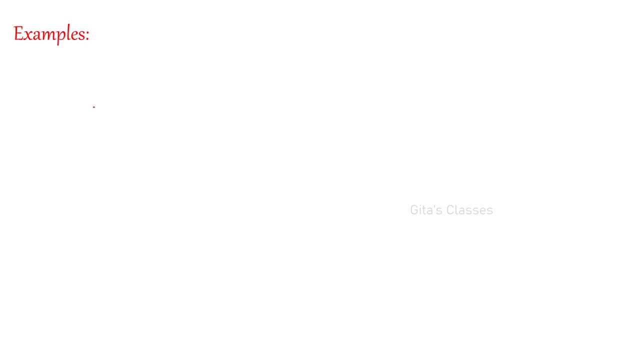 have any idea for that. So always domain should be mentioned. So there exists means for some. sometimes we will have different statements: there is and there for at least one, etc. So we will see some examples. There exists x, p of x. You try to find out whether it is. 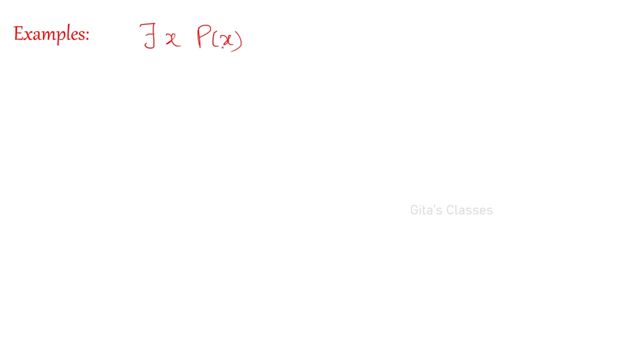 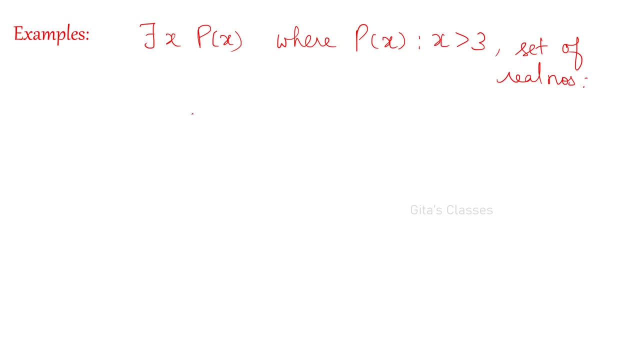 numbers. So can you find out at least one x in this set of real numbers, such that x greater than 3?? Yes, I can. x is equal to 5 is greater than 3.. Therefore, it will become true. Next, this is one example. second one: There exists x, q of x, where q of x is equal. 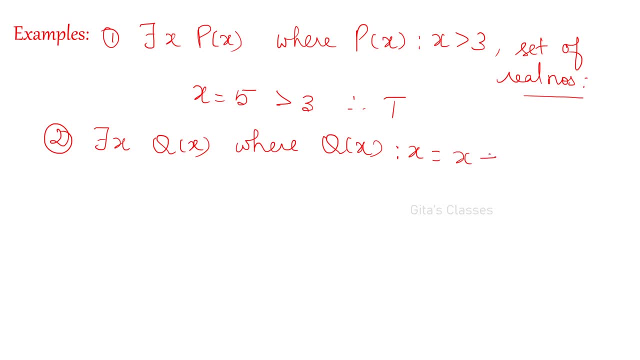 to x, p of x. So there exists x, p of x, where q of x is equal to x, p of x. So there exists. x is equal to x, p of x. So there exists x. p of x, so that x is equal to its p of x. So 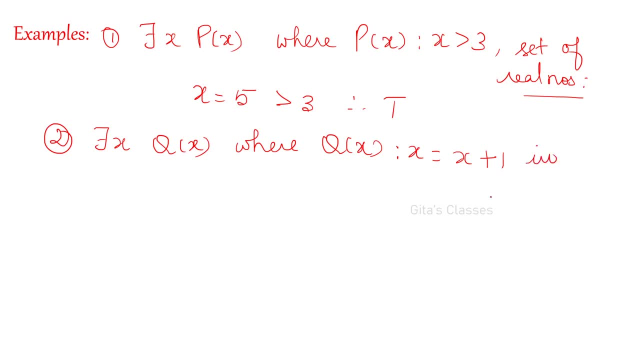 there is the question of getting p of x. Which p of x is equal to x p of x. The answer is x. p of x greater than zero to the power of indigenous escri Крас. So which p of x is greater than zero or minus nothing? M. Now this is the question. Which块 of black? 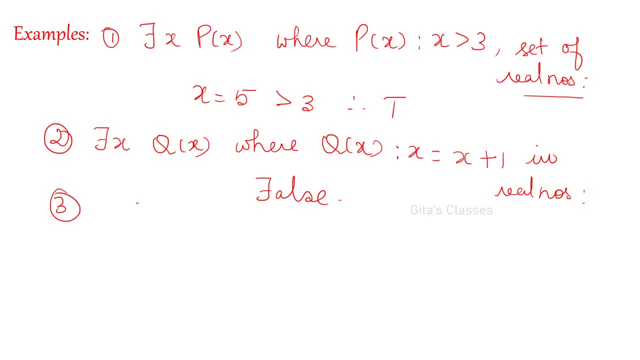 white is equal to z or z, equal to z minus nothing B. So here it is q or z greater. example 3: we have know. so for all, x, p of x. where p of x is x squared less than 10, we have, we have written this right. so if p of x is greater than or equal to- sorry, x squared is: 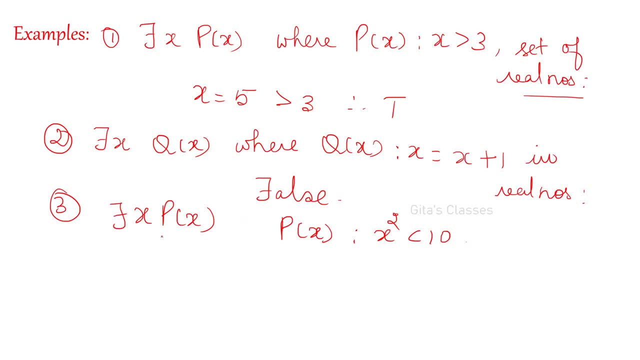 less than 10. there exists p of x. what will be the value of this now? p of x? is x squared less than 10? there exists some x where it is again set of the same domain. x is having the values 1, 2, 3, 4. 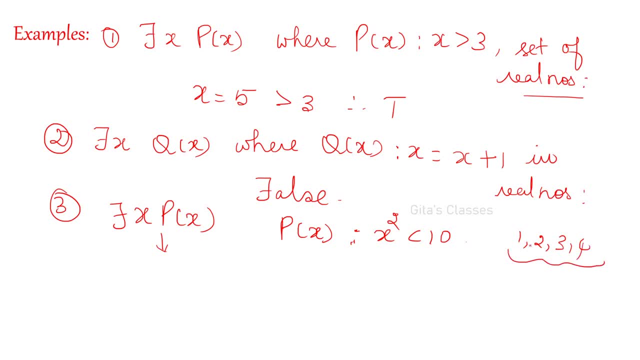 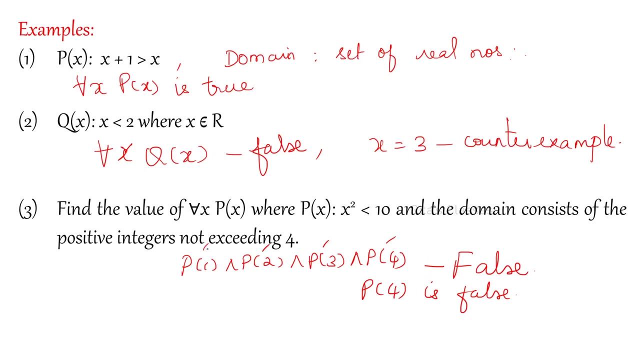 the domain is 1, 2. set of integers 1, 2, 3, 4. so if i have, there exists x. yes, we have 1, we have 2, we have 3, so it is true. so what we have defined in the previous one, this question, question number 3. 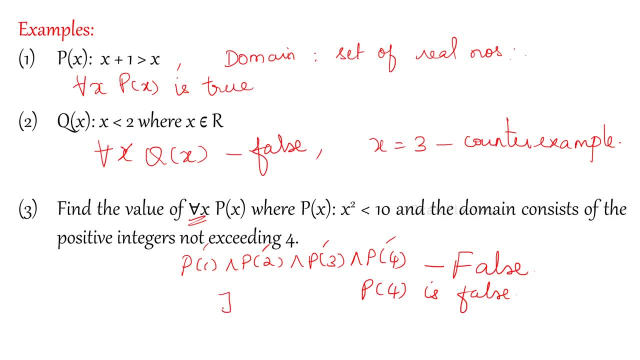 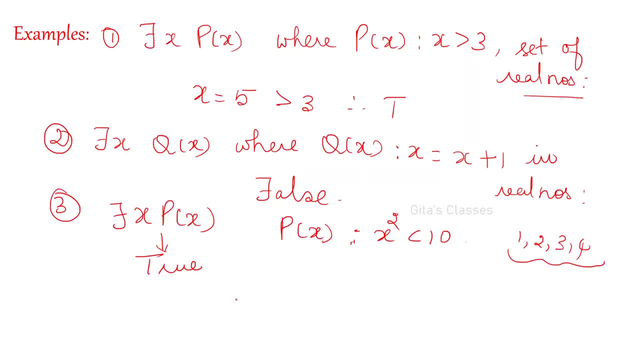 find the value of in the place of for all. if there is, there exists p of x, then it will become 2 here for all. p of 4 is false. therefore we have told that it is false. okay, so here we can give the example. at least one means so 1, 2, 3 for those. 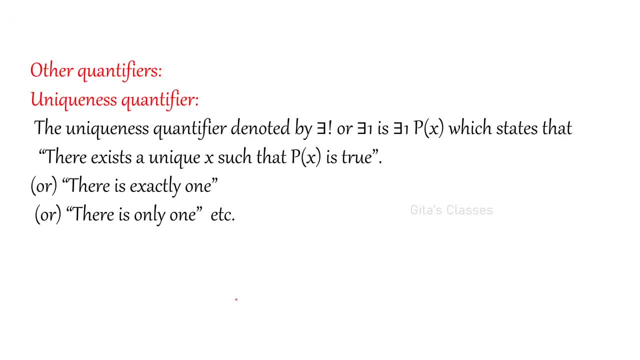 values, it is true. next is one more quantifier we don't use much, but sometime, uniqueness quantifier. uniqueness quantifier: we denote it by there exists, with this exclamatory symbol. or sometimes there exists one? okay, suffix one. so this is the uniqueness quantifier, p of which says: 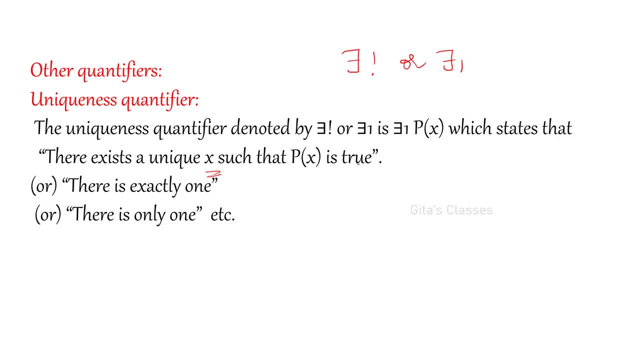 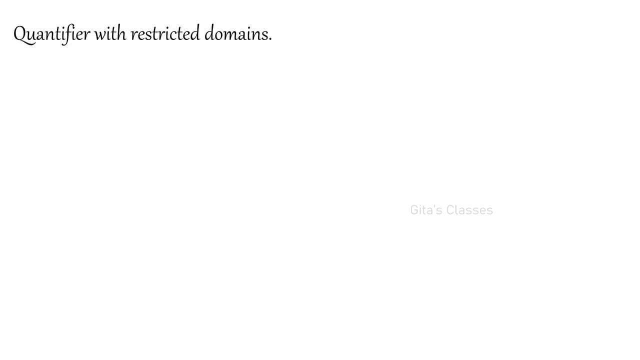 that there exists a unique x, such that p of x is true. okay, there is exactly one. there is only one value, then we use that, but we don't in practice. we don't use much in the in our practice, okay. next is quantifiers, with some restricted domains. i'll give you some examples here. 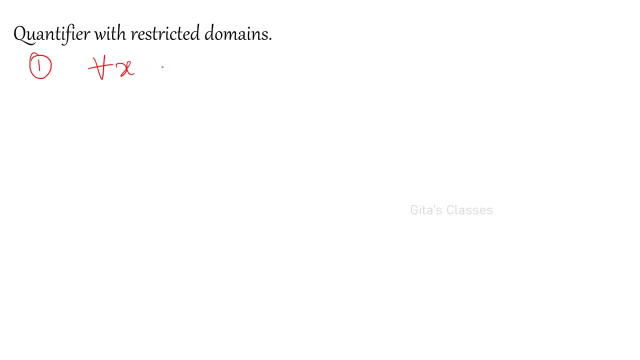 the statement: for all x less than 0 x squared is greater than 0. that is what the state said for every real number x. for every real number x greater than 0 x squared will be greater than 0. is it correct or not? for every x less than 0 x squared will be greater than 0. is it correct or not? yes, it is true, right. 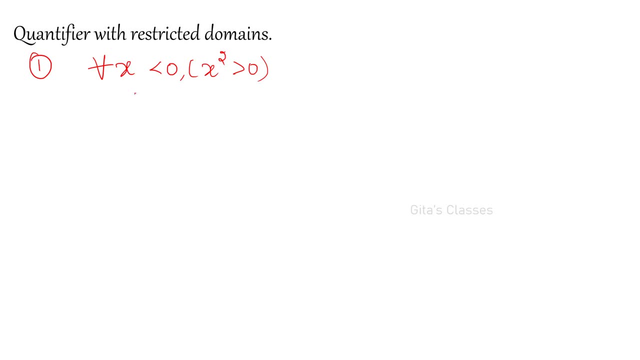 it is equal and true. that is, instead of writing this, what will be right, what you can write in the statement form: the square of a negative number, the square of a negative real number. here, for every real number you can say: domain is real, set of real numbers. 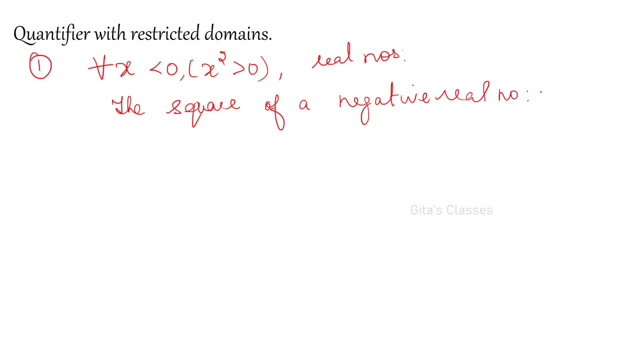 the square of a negative real number is always positive. okay, so one more example. i'll give you the. actually here, instead of writing p of x, q of x and all with restricted domains we have, we can write like this also for all x. instead of writing p of x, q of x, you can write like this or this can: 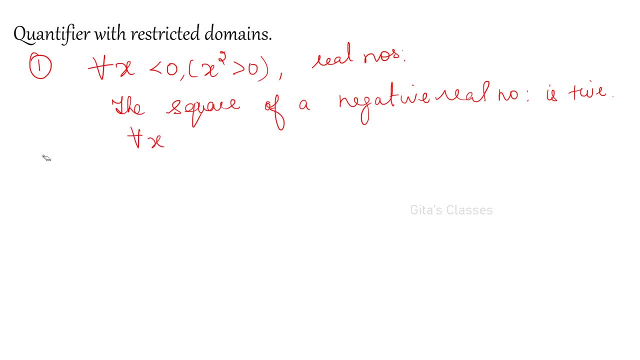 be equivalently. we can write this as for all: x, x less than 0. conditional x squared greater than 0. that is, if there is a real number with less than 0, definitely x squared is greater than 0. okay, this can be written like this. so we can write like this. so we can write like this. so we can write. 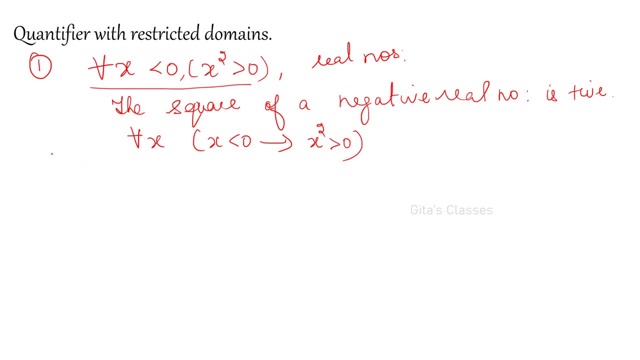 and equivalently like this also in terms of universal quantifier. similarly the next one: there exists z greater than 0 and z squared is equal to 2. how will you write this? there exists- is it that is what you mean by this? and here again, a set of real numbers only. 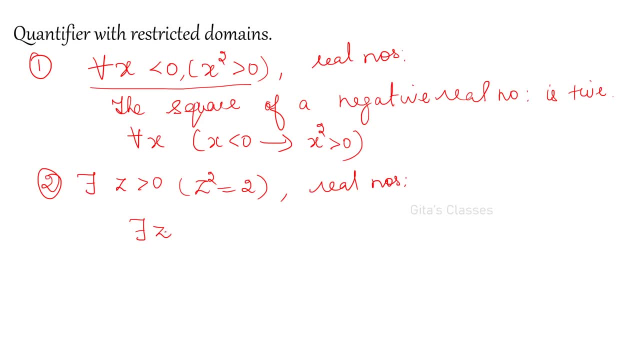 the domain is the set of real numbers, but there exists some value such that z is greater than 0 and z squared is equal to 2, so this is equal to 2, and z squared is equal to 2, so this is equal to 2.